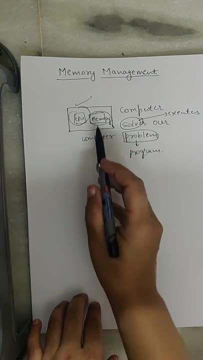 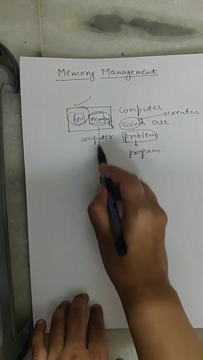 So here problem is stored And one by one CPU picks up the problem from memory and executes it, And this memory is nothing but a program, But main memory. We can also call it main memory, We can also call it physical memory, And we can also call it primary memory. 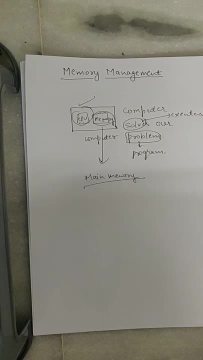 So what does operating system do? It manages the memory. Manage means we can efficiently use the memory And we can also efficiently use the CPU. Now, what will be the work of CPU? It will pick the program from the memory and execute the same program and give us the output. 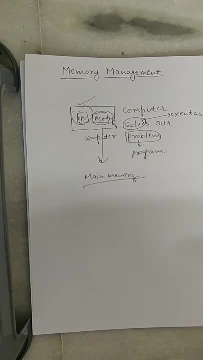 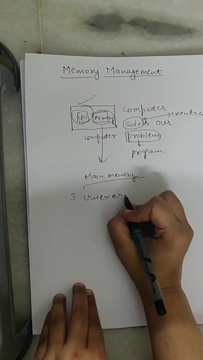 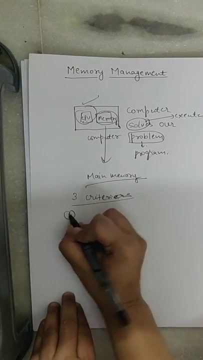 Which memory should we use for memory? What should be the criteria? We have to think about three criteria which are very important To choose any three criteria for memory. what should be the three criteria? First will be size. Second will be its access time. 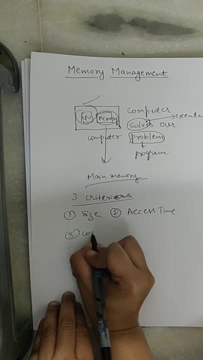 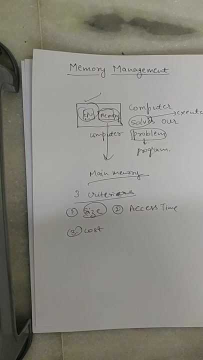 And the third one is cost. Okay Size means its size should be so big that our program should be there. Okay Size means its size should be so big that our program should be there And it should fit in that memory. What does access time mean? 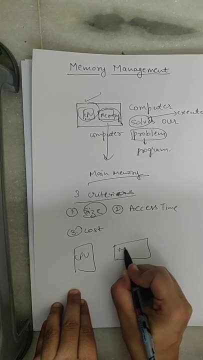 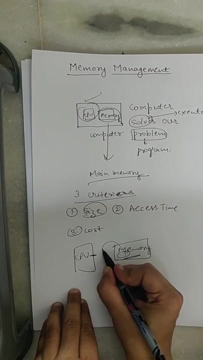 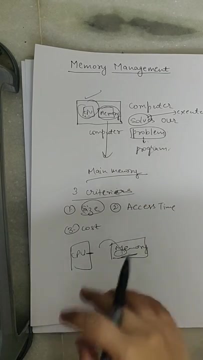 What I said is CPU and this is memory. Okay, There are programs in memory, So access time means when CPU picks the program from memory, then in that case it should take less time. Okay, When CPU picks the program from memory, then its total time period should be less. 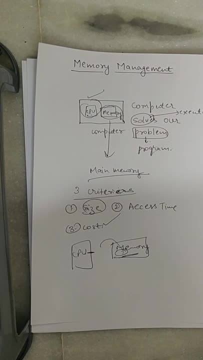 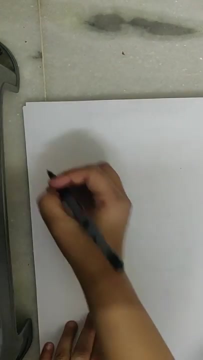 This is access time. Third is cost: Memory should not be expensive. Okay, So these are the three criteria which we should keep in our mind before choosing any memory. Okay, Now let's see what type of memory we actually have. What happens is we do memory hierarchy. 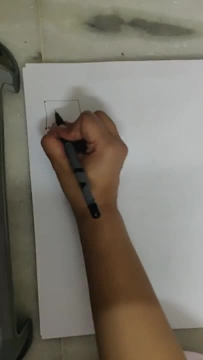 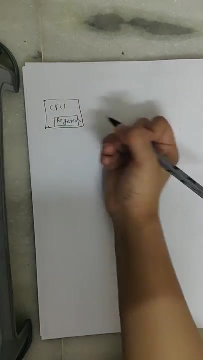 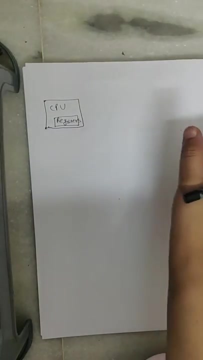 Okay, From where memory comes from, How, How? This is CPU. So there is memory inside CPU. Okay, That memory we call registers. Okay, Now I will explain these memories one by one. For now, let's see where actually memories reside. 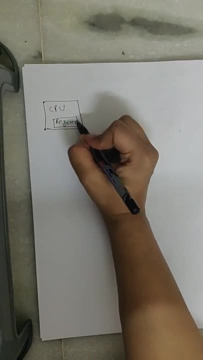 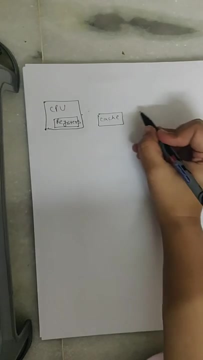 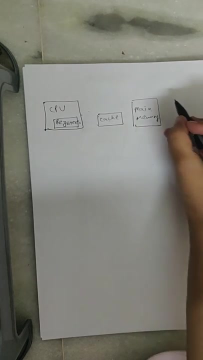 Okay, There are registers inside CPU. Okay, A little bit away from that is cache memory. I will discuss all these memories. Okay, There is cache memory. A little bit after that is main memory. Okay, There is main memory. And then in the last, farthest from CPU. 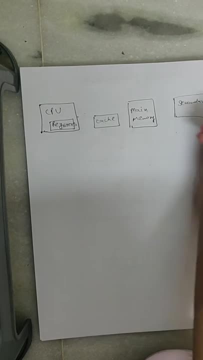 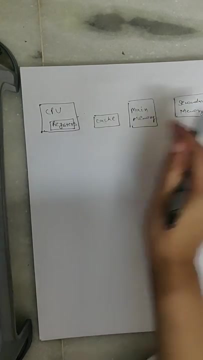 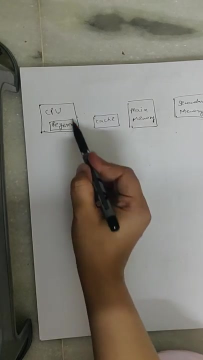 Okay, There is secondary memory, Like your hard disk, pen drive, magnetic tape, magnetic disk, Secondary memory- Okay. Now, if we talk about size, then the size of registers memory inside CPU is very less. Okay, Registers is a memory, but it is a temporary storage whose size is very small. 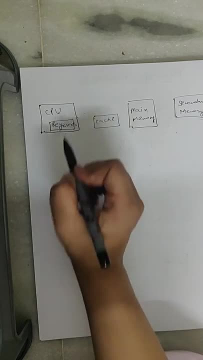 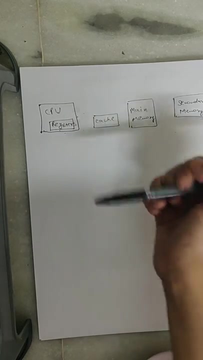 Okay As compared to other three memories, But access time is very fast. I have just discussed access time. Access time means how much time does CPU take to pick any program from memory? Now, the obvious thing is that there are registers inside CPU. 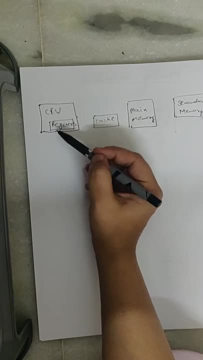 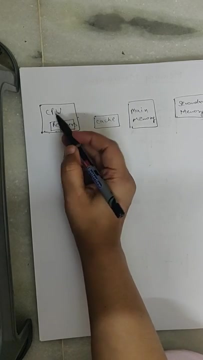 So access time will be less. Okay, So this is an advantage that access time is less, But the disadvantage is that the size of registers is small. So its size is small, but its access time is fast Because CPU can easily pick how much is its pass. 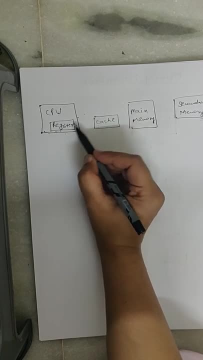 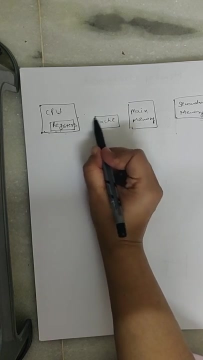 Next is cache. Comparatively, cache's access time is less than registers, but it is more than others Because it is a little closer to it. Okay, So in cache memory we keep those programs which are used recently. Okay, One is program 1,, program 2,, program 3.. 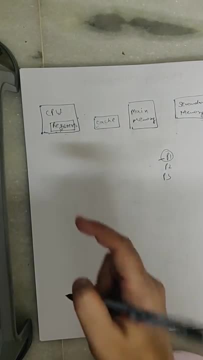 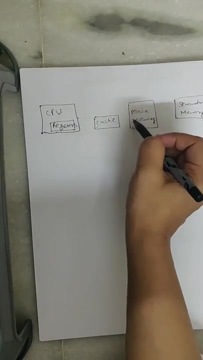 Program 1 is being used repeatedly, So we put it in cache memory. Why do we do this? Because access time for CPU is fast As compared to main memory. Because main memory is far, So the access time of the CPU is more. 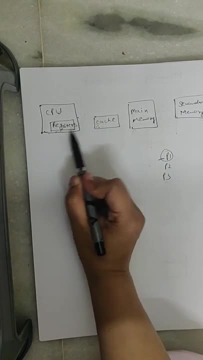 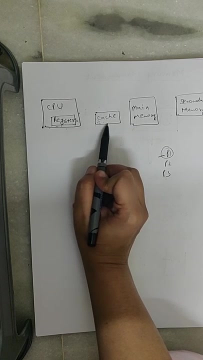 If we compare the size of registers and caches, then the size of registers is smaller and compared to caches the size of registers is bigger But the access time of registers is more as compared to caches, Because caches are a little far from CPU. 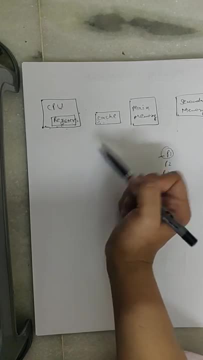 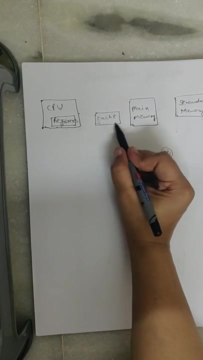 Okay, And in caches we keep the programs which are used recently. Okay. Next is main memory. If we compare, if we talk about size, then the size is slightly larger than caches and larger than registers. The size of main memory is bigger than registers. 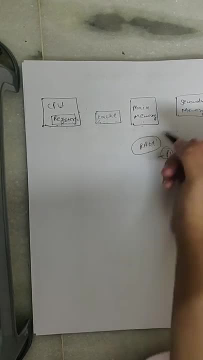 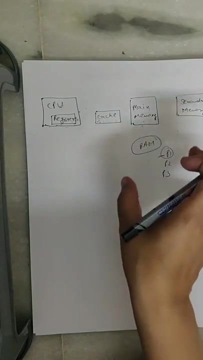 Main memory is nothing but your RAM. Okay, So main memory directly accesses the CPU. Okay, All the programs which have to be executed in RAM, they reside in the main memory. CPU directly accesses the main memory. First of all, what does it do? 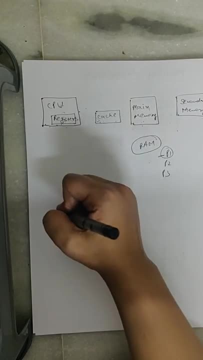 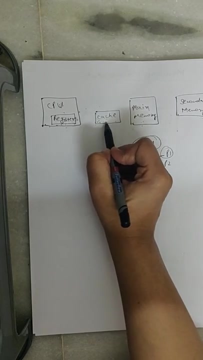 CPU checks in registers. Say suppose it has to execute program 1, then it will check in registers first. If it will not get in registers, then it will check in caches. Okay, If it will not get in caches, then it will check in main memory. 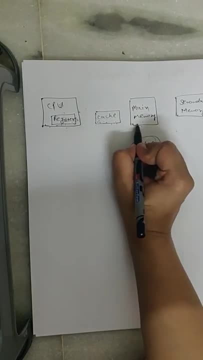 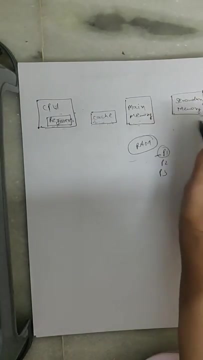 Okay, So main memory is nothing but RAM And the size of main memory is slightly larger than caches. Okay, Next is secondary memory. Secondary memory is permanent storage. This is temporary RAM is temporary. As soon as we power off the computer, RAM gets empty. 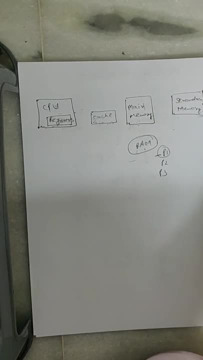 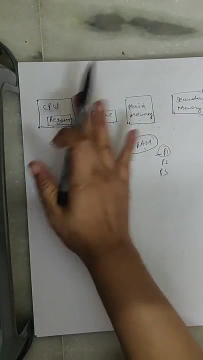 Next is secondary memory. Secondary memory is nothing but your hard disk, pen drive, magnetic tape, magnetic disk. This is all secondary memory, So it is far away from CPU And CPU can't directly access it. So suppose there is program P1 in the secondary memory. 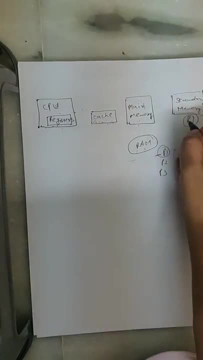 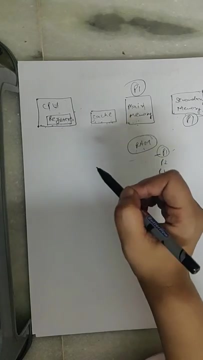 So if we want to execute program P1, then it has to be inside the main memory. It will shift from the secondary memory to the main memory Only after that it can be executed. Okay, So let's see with an example. 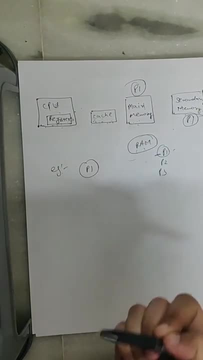 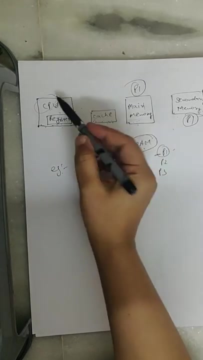 Suppose I have to execute P1.. We have brought P1 in the main memory. Okay, So CPU will check in registers first. If it didn't get P1, then it will check in cache memory. If it didn't get P1 in cache memory, then it will check in main memory. 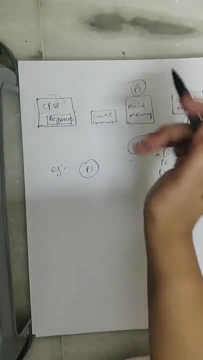 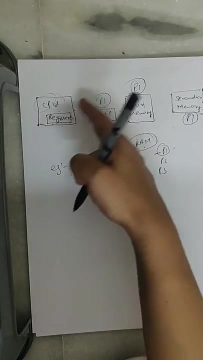 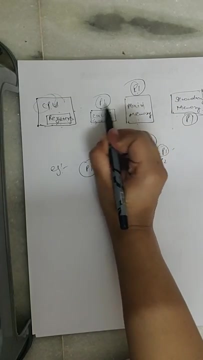 After that, after the execution is completed, it will keep P1 in cache So that next time when CPU has to execute P1, it will check in cache and get P1.. So, as I have already said, recently used programs reside in cache memory. 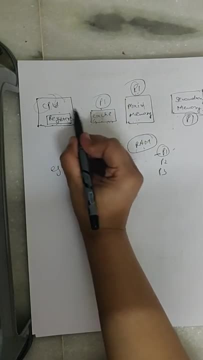 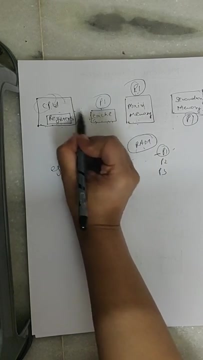 So why did we keep P1 in cache? So that the access time becomes fast. It doesn't have to go back to the main memory and access it. Because the access time of cache is fast. Okay, Because it is near the CPU. 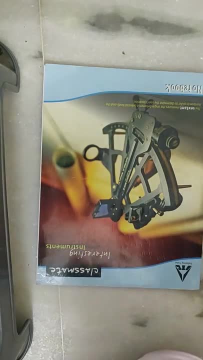 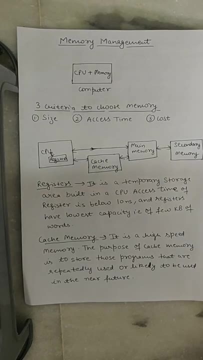 Okay. So let's see the notes of this. You can take the screenshot of these notes, Okay. So, if you want, you can take the screenshot. You can take the screenshot by pausing. So this is. I have already discussed all this. 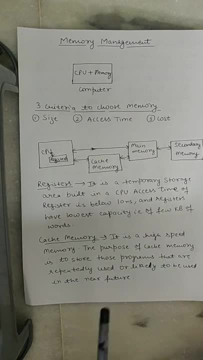 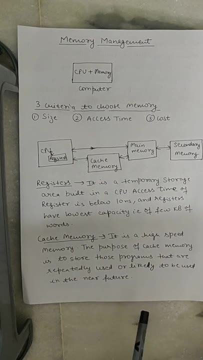 Registers is a temporary storage: Okay, It is built inside the CPU And this is high speed memory, Okay. High speed means its access time is fast. To store the programs that are repeatedly used: Okay, And we feel that they are going to be used in the near future. 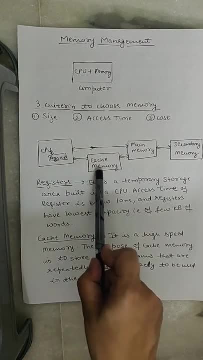 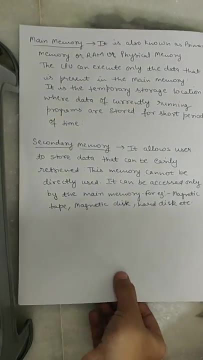 So we keep it in cache memory, So that the CPU takes less access time, So that it doesn't have to use more time to go to the main memory. Next is main memory is nothing but RAM. Okay, This is RAM Okay. 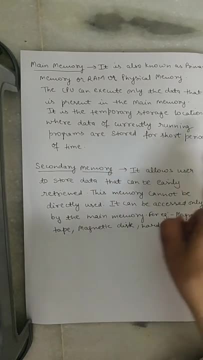 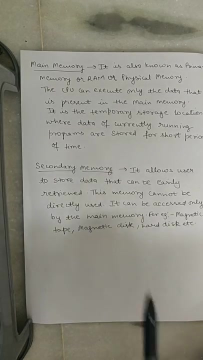 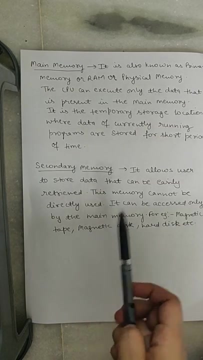 And we call it physical memory too. CPU can execute this memory directly. Okay, And we call this temporary storage location, too, Where programs reside for a short time. Next is secondary memory. These programs are permanently stored here, And this memory cannot be directly accessed. 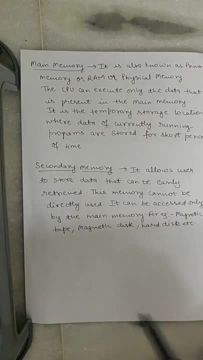 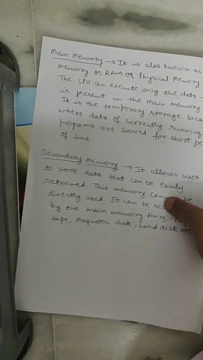 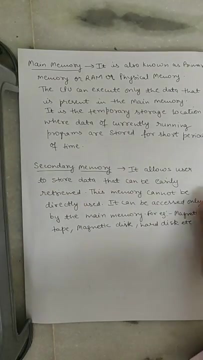 And there are examples of this Tape, magnetic tape disk. I have already discussed. You can take the screenshot. Okay, guys, This is a theoretical topic, So you can take a screenshot of this. I will adjust this. Okay, So you can take the screenshot of this notes. 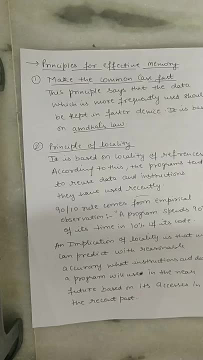 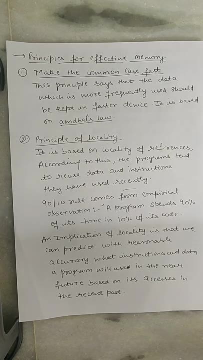 Now the next topic is principles for effective memory. Principles for effective memory: Okay. First one is make the common case. fast Means we want to use the memory effectively. So there are two main principles that we have to keep in mind. First one is make the common case fast. 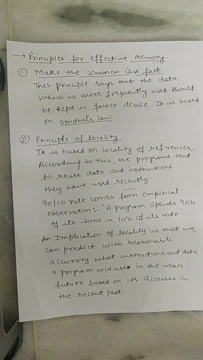 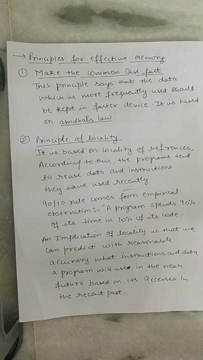 This means that the programs that are frequently used Keep them in a faster device. Faster. Just now we saw that program P1 was executed And it is being used again and again. CPU is accessing it again and again, So rather than keeping it in secondary memory or main memory, 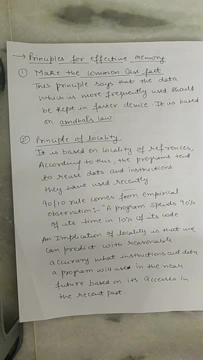 Keep it in cache memory Or keep it in registers if its size is small, So that it can be accessed fast. So make the common case fast. It is based on Amdahl's law. Second one is principle of locality. Principle of locality is based on locality of reference. 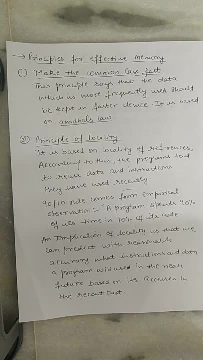 This means that what happens in your program? There is data and instructions. Okay, So the instructions that are being used again and again. Keep them in cache memory or main memory. This is based on 90 by 10 rule. This means that the program spends 90% of its time. 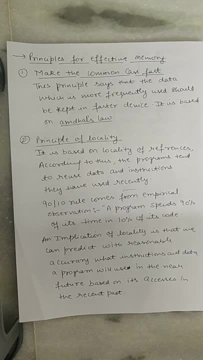 To execute 10% of its code Means You have a code, Okay. So CPU is giving its time to access that code. 90% Means it checked in registers first, Then checked in cache, Then checked in main memory. It didn't find that program anywhere. 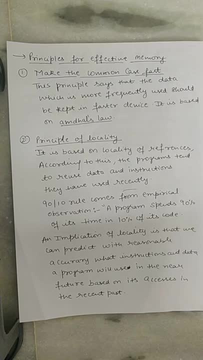 So we brought it from secondary memory to main memory, Then it was accessed there. Then next time it Means Only 10% is the code Okay, But we wasted so much time on it 90%. So This thing we have to keep in mind. 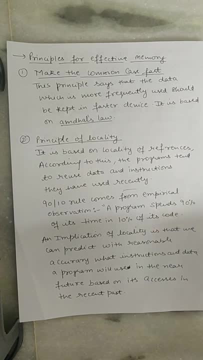 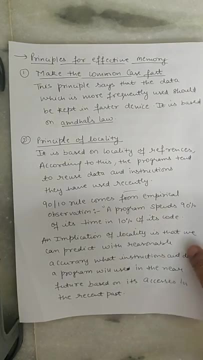 That the program, The data Or instructions That are being accessed again and again Keep them in cache memory. Okay, These are of two types. You can also take the screenshot of this, Okay, So These are also of two types. 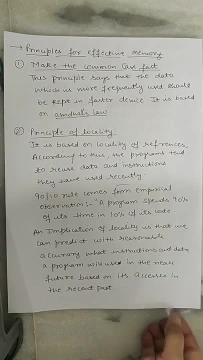 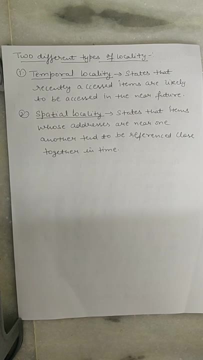 First is temporal. What is said in temporal? That the recently accessed items. Okay, Keep that Main memory, Okay. So This is also of two types. First is temporal. What is said in temporal? That the recently accessed items. 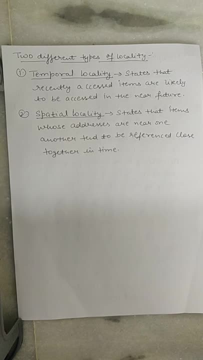 Okay, Keep that Main memory. Keep that Main memory Or cache memory, Which you think can be accessed in the near future. Okay, And the second one is spatial locality. You Nearby Say, suppose Data. Whatever our program is, 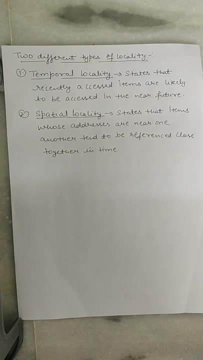 It will have addresses. Instructions will have addresses. So Say suppose There is an instruction on a thousand address, So Nearby, 99. 9999. And 1001. 1002.. Nearby The instructions of the addresses. 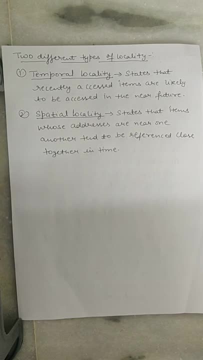 They Also Keep that In the main memory, Or cache memory, Because, Based on its Previous Execution Means, You Must know That you have already accessed the program P1. Once Okay, Next time, When that process, 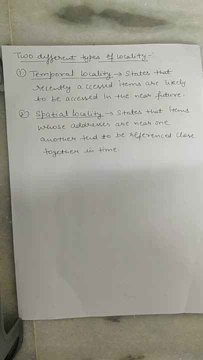 Cpu Accesses it. So You have to keep that in mind. That first. That means Say, suppose The instruction on a thousand address Was being used more So Nearby Addresses 99. 9999.. 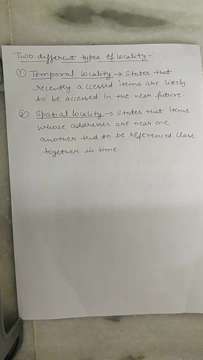 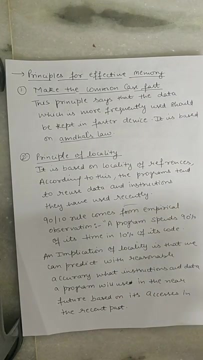 And 1001.. 9999. And 500. And 600.. 99.. 9999. And 500. And 109. And 1001. And 1002.. So 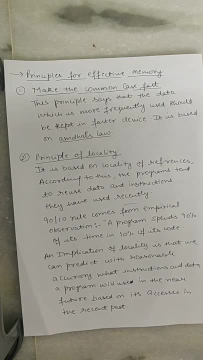 You Don't do anything, Okay, So Thanks For watching my video. Please Subscribe And Like. 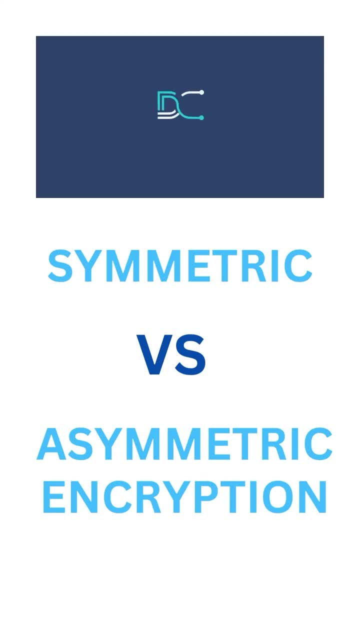 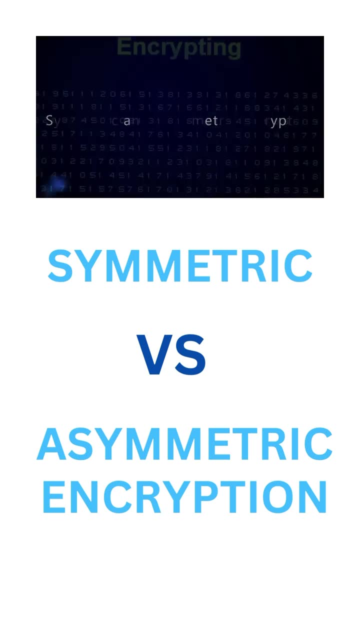 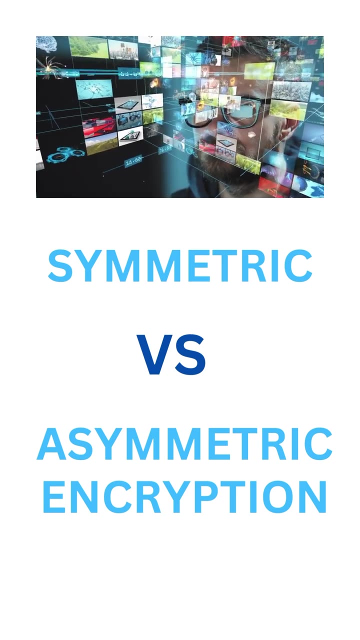 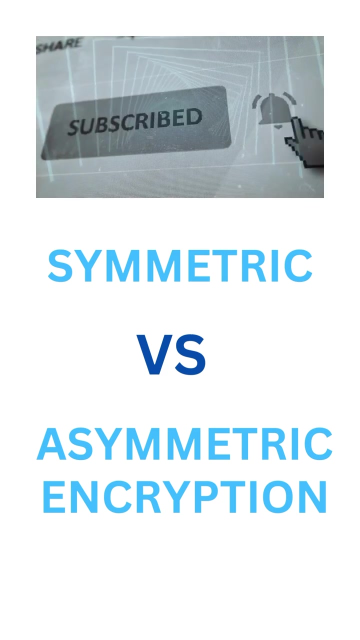 Welcome to Dallasiber. In this video, we dive into the world of encryption and explore the differences between symmetric and asymmetric encryption. Join us as we demystify the concepts, discuss their applications and help you understand how these encryption methods can safeguard your sensitive data. Don't forget to subscribe and hit the notification. 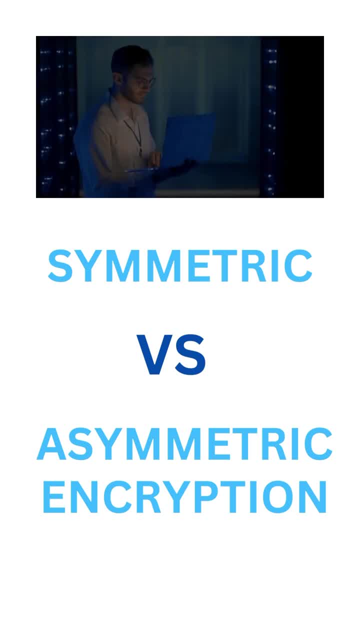 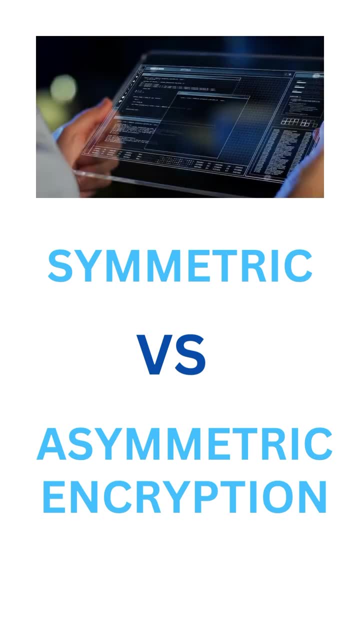 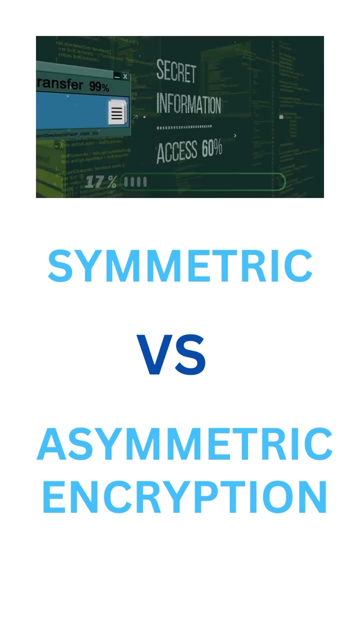 bell to stay updated with our future content. Welcome back to Dallasiber, your ultimate destination for everything related to cybersecurity and data protection. In today's video, we'll be tackling a fundamental aspect of encryption: symmetric versus asymmetric encryption. Encryption plays a crucial role in securing our data. 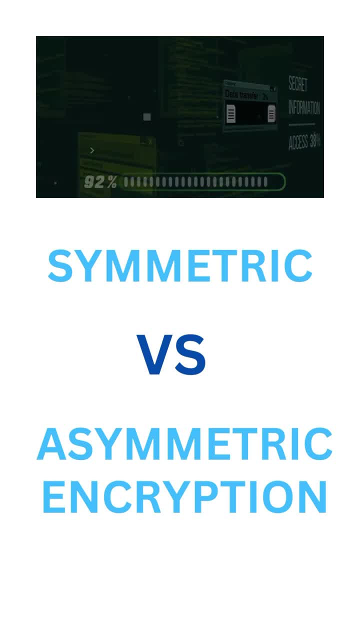 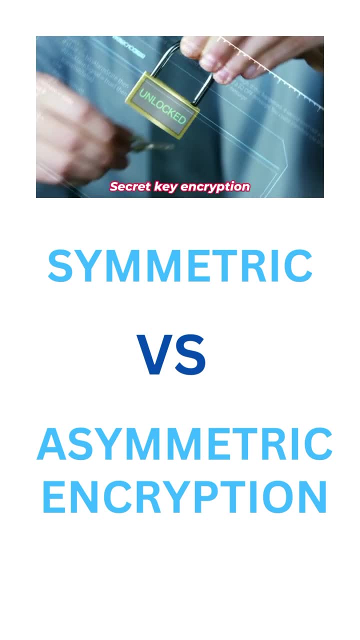 and understanding these two methods is essential in today's digital landscape. So what exactly is symmetric encryption? Symmetric encryption, also known as secret key encryption, relies on a single shared key for both encryption and decryption. This means that the same key is used to lock.